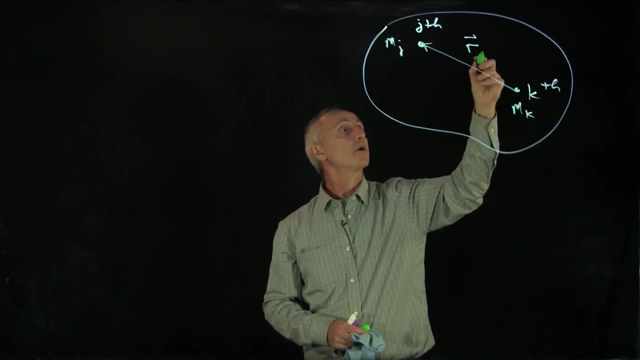 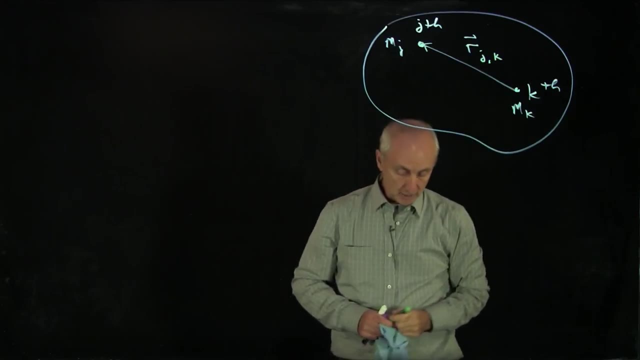 from the k-th particle to the j-th particle. So we'll draw that as rjk And actually I would like to write it from the k-th particle to the j-th particle. So we'll draw that as the third factor And we'll call that rkj And we're going to give it a function. 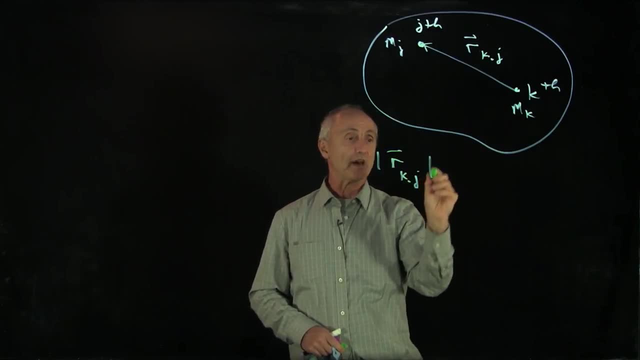 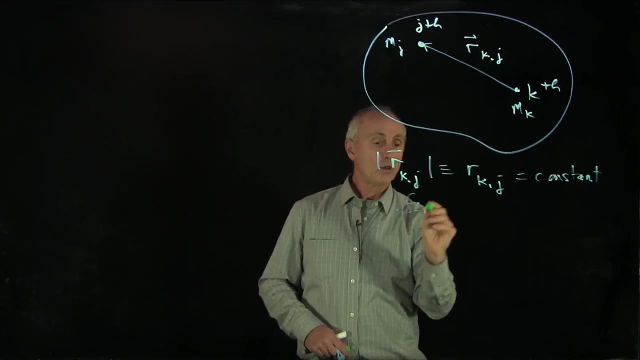 because we need the second function now, So we'll give it this function. So let's just say: Yes, You've already written rkj as the distance between the rigid body and the k-th point. Let's just write this function and I'll give it a function. So let's just say: rkj- second function minus kj- to the third particle, because we'll notice this direction. it has a similar resistance, So I'll create another condition. It's called the reliance on the j-th point. by rotating theOL from the인 particle to thepj-th particle, rkj And 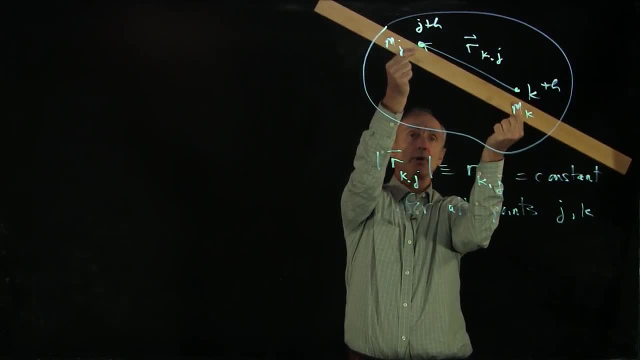 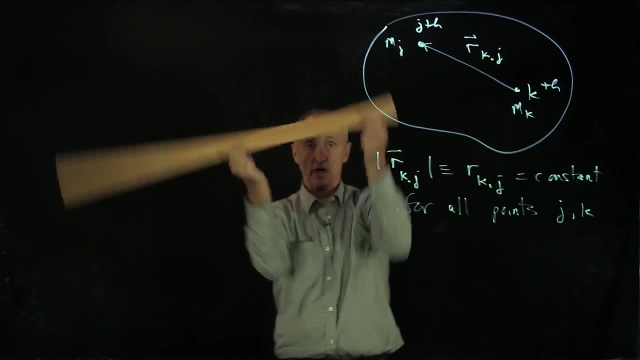 our condition is that the magnitude of this vector, which I'll denote as rkj, is constant for all points j and k. Now, what does two points in the rigid body stays fixed, no matter how the rigid body is moving and no matter what two points I choose. 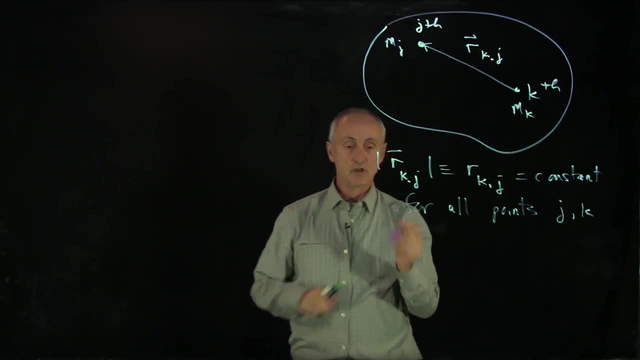 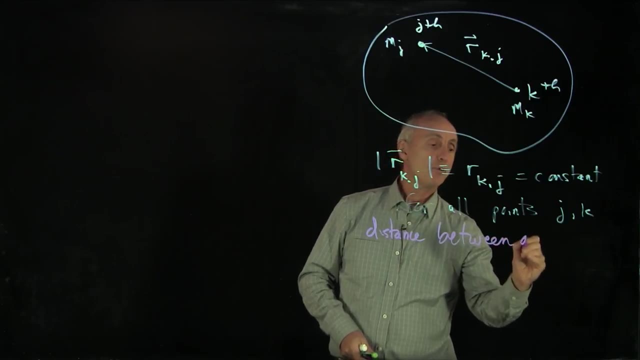 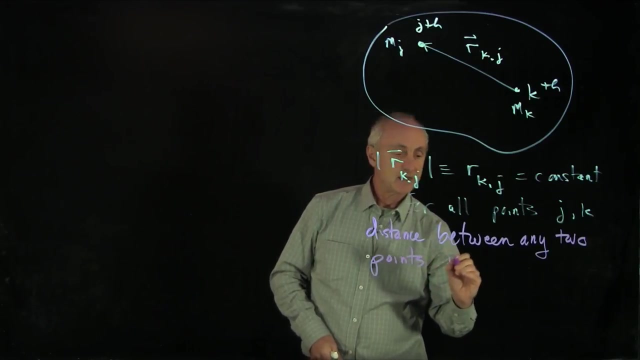 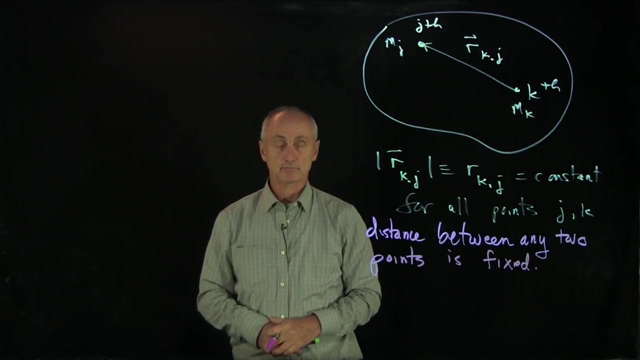 the distance between any two points is fixed. So we'll rewrite this as the distance between any two points is fixed, So that doesn't change, And that's what we call the rigid body condition. 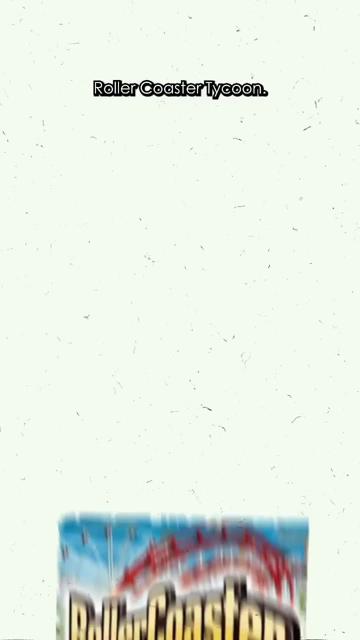 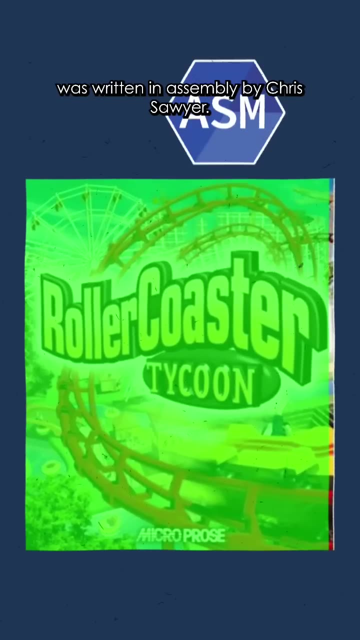 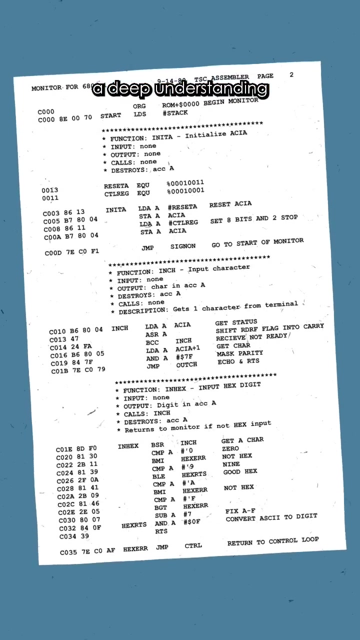 This game was written in one of the hardest programming languages. Rollercoaster Tycoon was released in 1999 and was amazing. 99% of the code was written in assembly by Chris Sawyer. Okay, what is assembly and why is it so hard? Assembly requires a deep understanding of the machine and 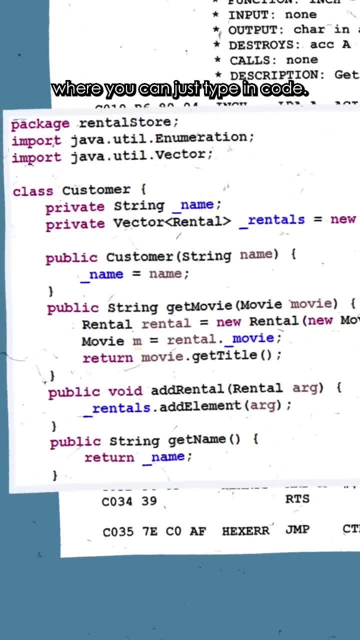 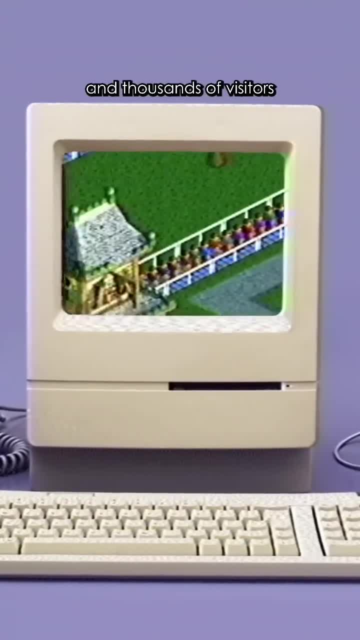 CPU you're working on, unlike most programming languages where you can just type in code. Because of this, Sawyer was able to make the game, render in-game economies, roller coasters and thousands of visitors at the same time. Overall, he made over $30 million. 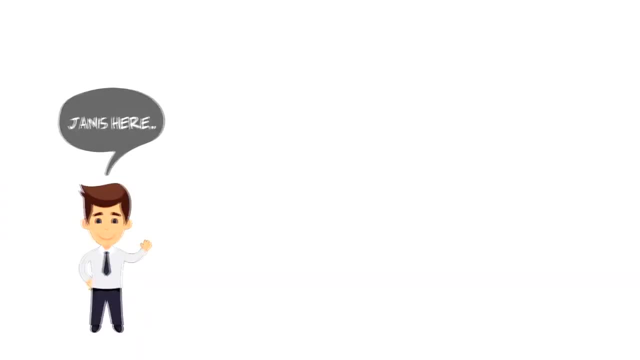 Hi everyone. it's Yanis here, and in this video we will explore what is deductive reasoning. To make better decisions, it is important to use validated information instead of guessing and hoping. If this is your first time on this channel, then make sure you subscribe and hit.